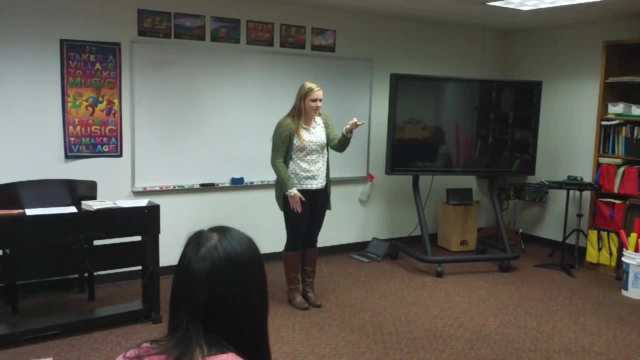 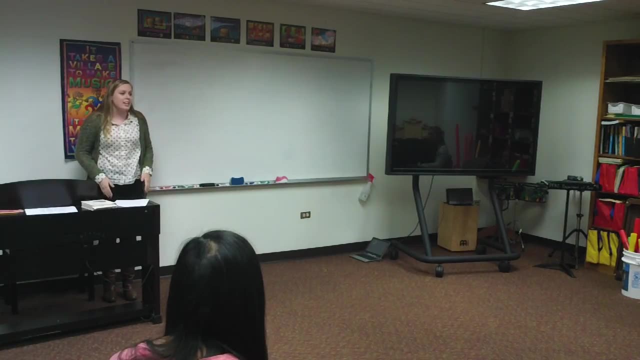 We're all here together again. Wonderful job class. Okay, we are going to sing a song that you should already know, So I'm going to start singing it, and when you feel like you know it, you can join in. 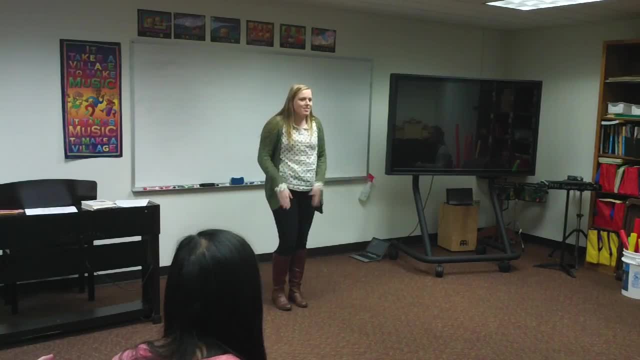 A-rim-sim-sim. A-rim-sim-sim: Gooly, gooly, gooly, gooly gooly. Ram-sim-sim. A-Ral-fi, A-Ral-fi, Gooly, gooly, gooly, gooly gooly. 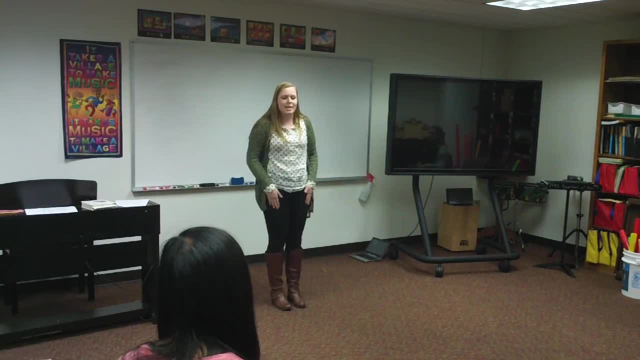 Ram-sim-sim A-Ram-sim-sim- A-Ram-sim-sim. Gooly gooly, gooly, gooly gooly. Ram-sim-sim A-Ral-fi- A-Ral-fi. 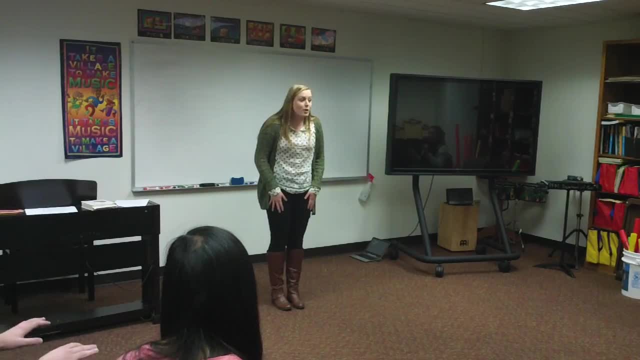 Gooly, gooly, gooly, gooly, gooly, Ram-sim-sim. Great job. Okay, we're going to sing it again and I want you to follow me, okay, A-Ram-sim-sim, A-Ram-sim-sim. 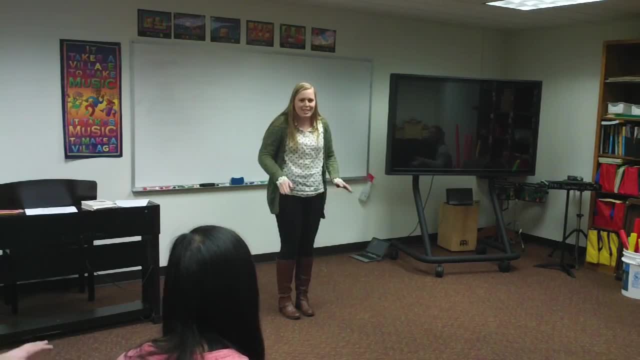 Gooly, gooly, gooly gooly Ram-sim-sim. A-Ral-fi. A-Ral-fi. Gooly gooly, gooly gooly Ram-sim-sim. Great job, Okay, one more time, Follow me. 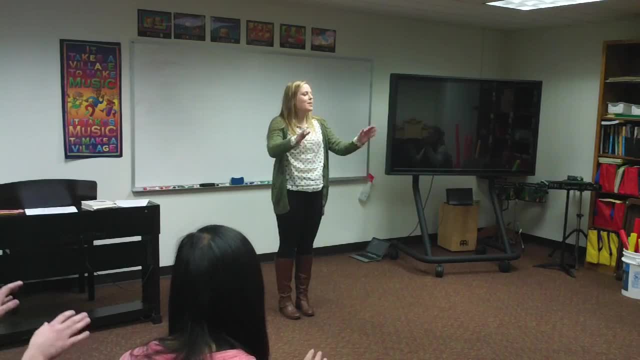 A-Ram-sim-sim. A-Ram-sim-sim: Gooly, gooly, gooly, gooly gooly. Ram-sim-sim. A-Ral-fi. A-Ral-fi- Gooly, gooly, gooly, gooly gooly. 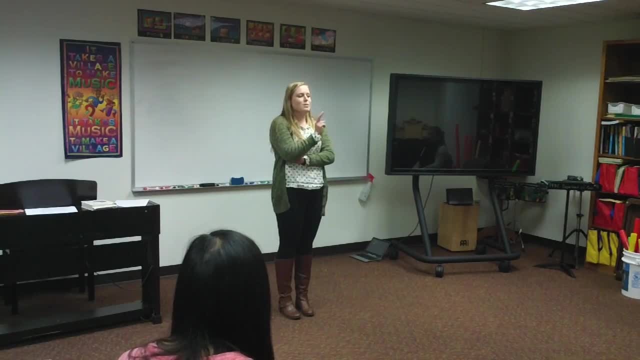 Ram-sim-sim? Were those two times we sang that song the same, or were they different? Different? They were different. Great, Now can someone raise their hand and tell me how they were different? Hannah, The first one was really fast and the second one was really slow. 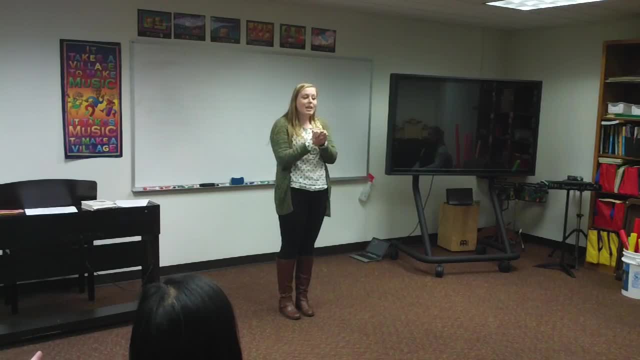 Yes, the first one was really fast and the second one was really slow. Today we are going to be learning about music that can be really fast or really slow, and we're going to learn a new word for our word wall today. 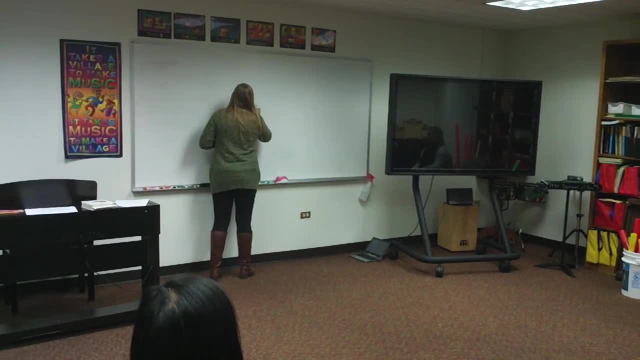 and that word is tempo. Can you all say it with me? Tempo? Now, tempo means the speed that the music gets, whether it's fast or it's slow, And so we are going to look at something that you guys are also familiar with. 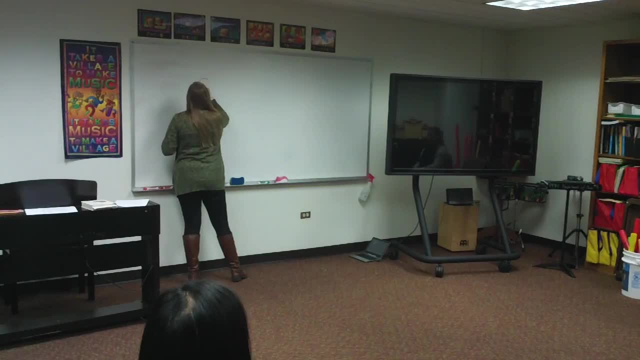 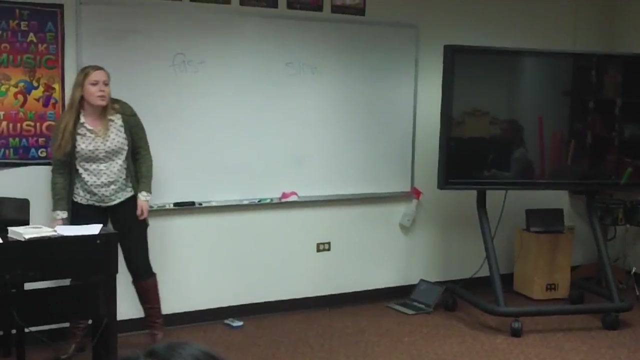 I'll put that up later at the end. So we have fast over here and slow over here. Who here likes animals? Yes, Okay, Now I'm going to show you guys a few animals and I want you to take a few seconds to think to yourself at first. 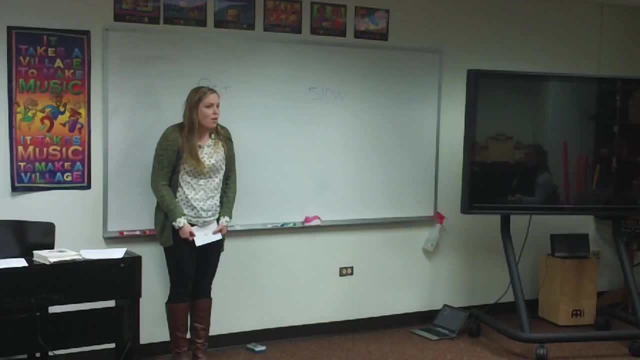 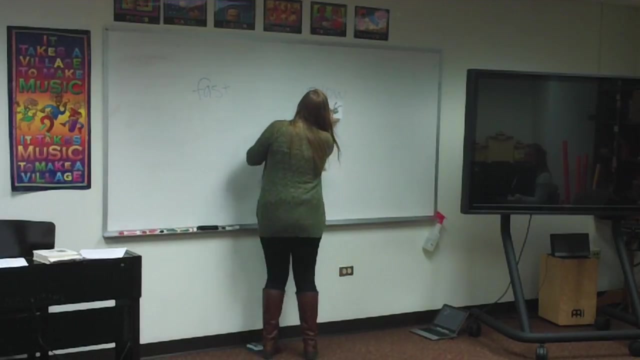 whether this animal is fast or slow, and then, when I ask you, you can tell me the answer: okay, Is a snail, fast or slow? Think to yourself for a second. Fast or slow, Slow, Good job, So we're going to put it under slow. 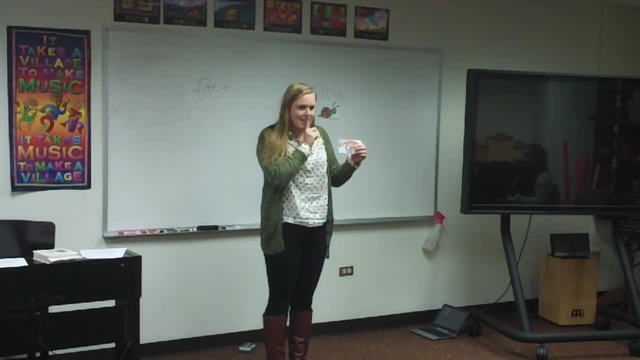 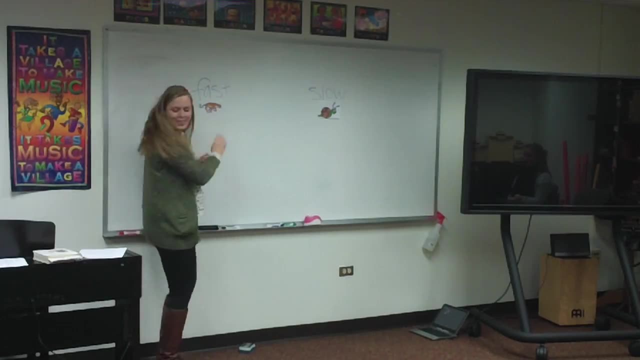 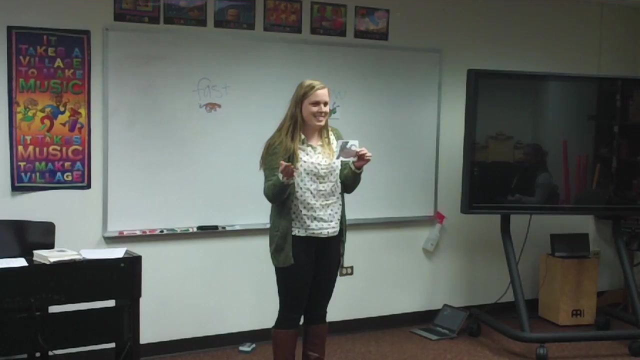 What about a cheetah? Think for yourself for a second. Is it fast or slow? Fast, Yes, it's fast, Good job. What about a sloth? Fast or slow, Slow, Slow, Very good, Slow, Thank you. 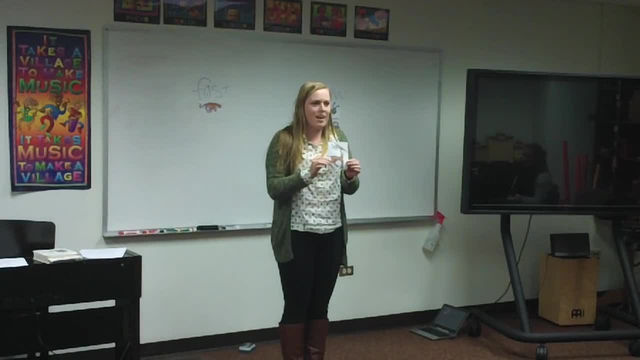 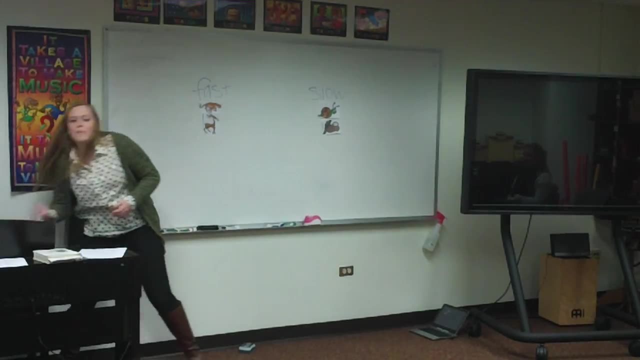 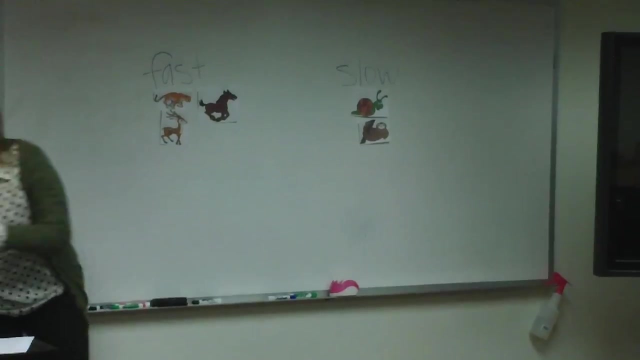 You guys are on it today. What about a deer? Is it fast or slow, Fast, Fast, Yep. What about a horse? Fast, Fast, right, And one more: we have a turtle: Slow, Slow, Good job. 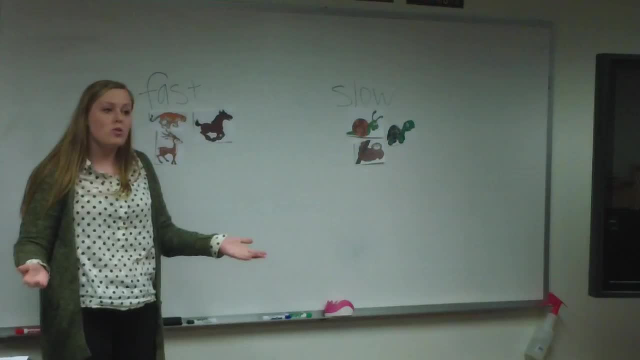 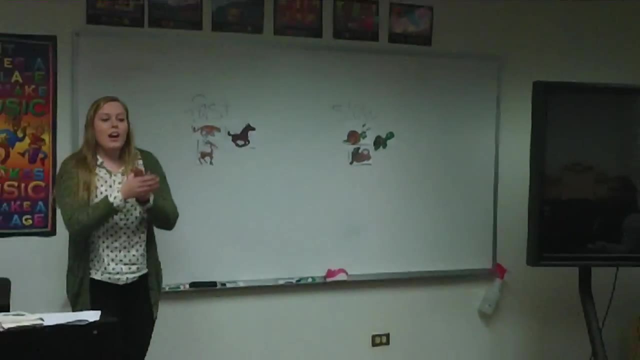 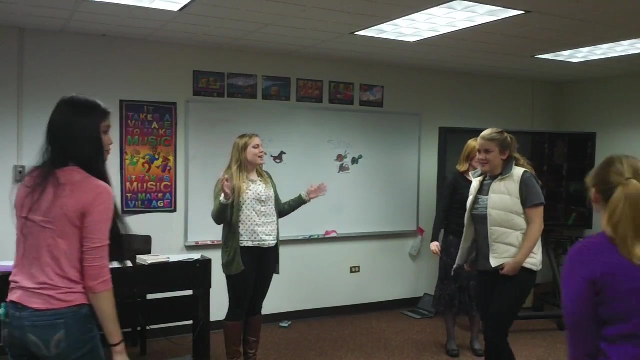 So, just like our animals can be fast or slow, our music can also be fast or slow, And so we are going to all stand up and find our own place in the room. This is my place, this is my space, my place, my space, nobody but me. 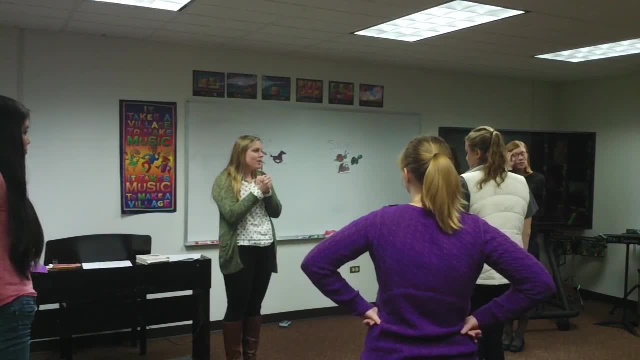 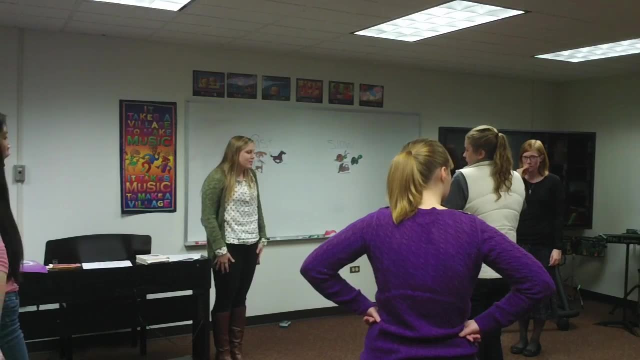 Awesome job. So we need to be very respectful and not hit our friends. We can move around if we want to during this activity, but we need to always keep our hands to ourselves. So what we are going to do now is you are going to hear a piece of music. 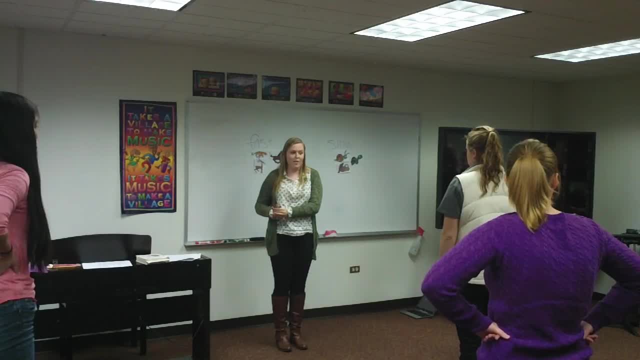 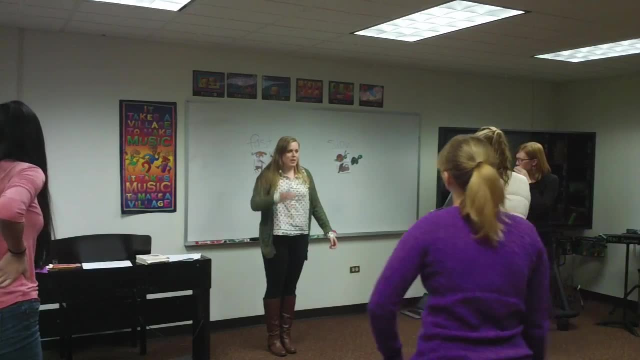 And it's either going to be really fast or really slow. And so when you hear fast music, I want you to dance crazy, really fast, really fast. And then when you hear slow music, once you move really slowly you can do some ballet really slow. 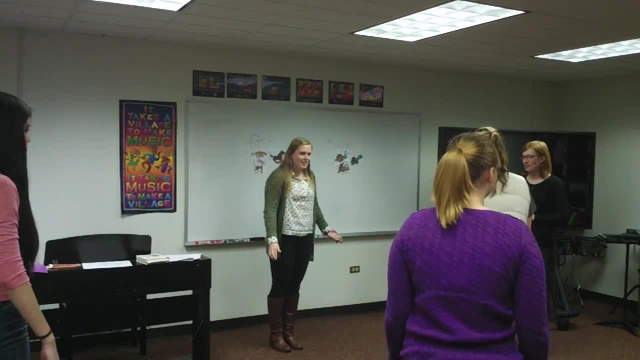 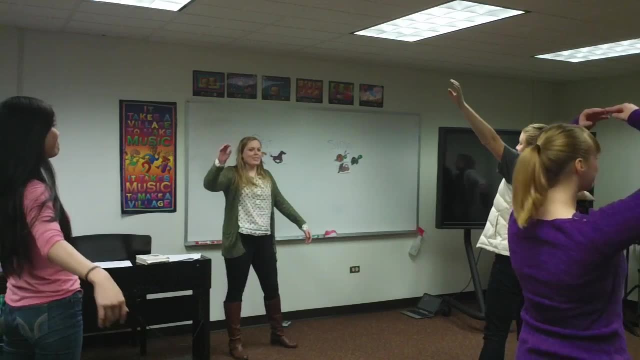 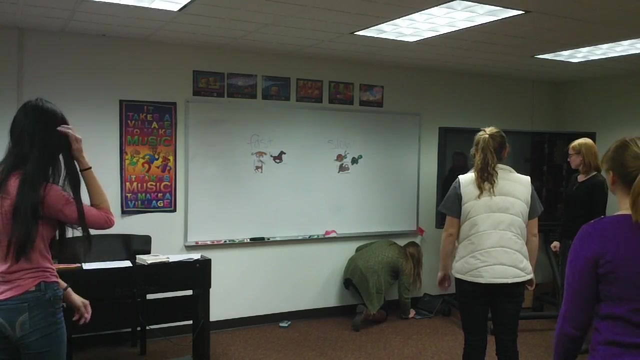 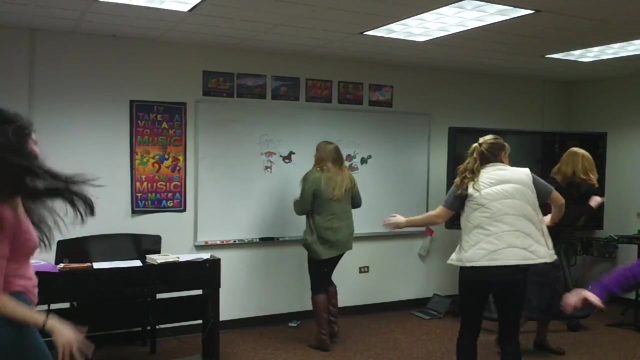 So can you all show me what your fast dancing is going to look like? Awesome. Now show me what your slow dancing is going to look like- Great job. Alright, now let's listen to this first one. Great job, That was fast. right, That was very fast. 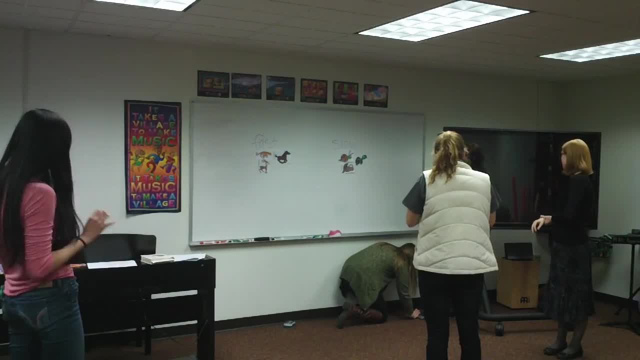 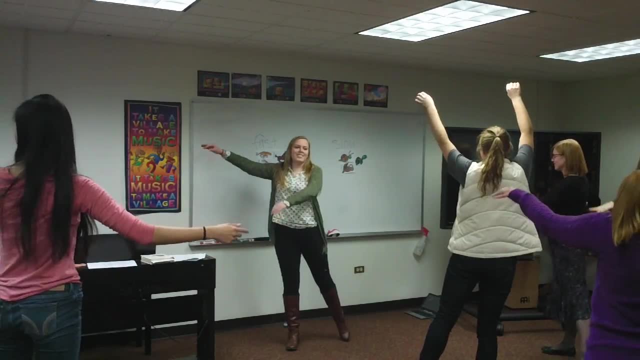 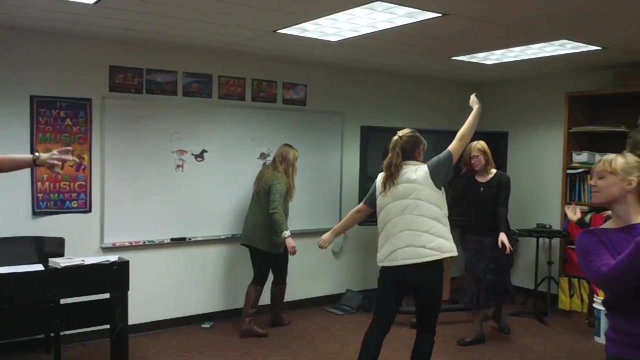 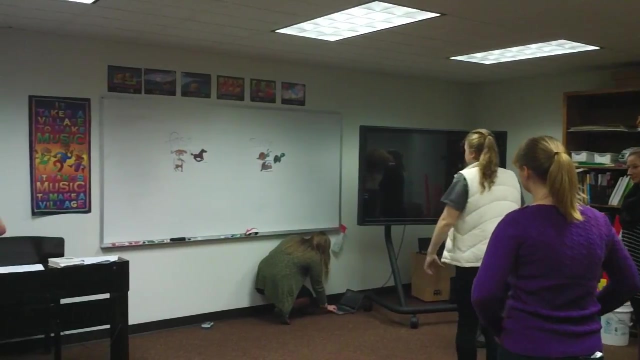 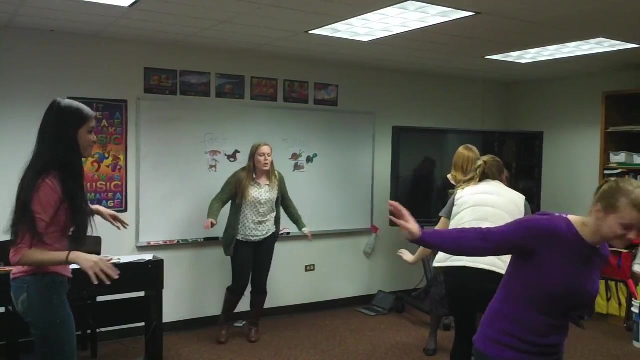 You guys got that all on the first try. Now let's listen to another one. Good job, This is slow, right, Very slow. Alright, let's try another one Very fast. What animal or bug do you think this might sound like? 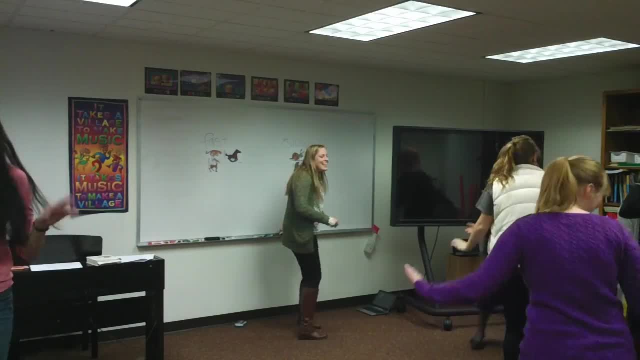 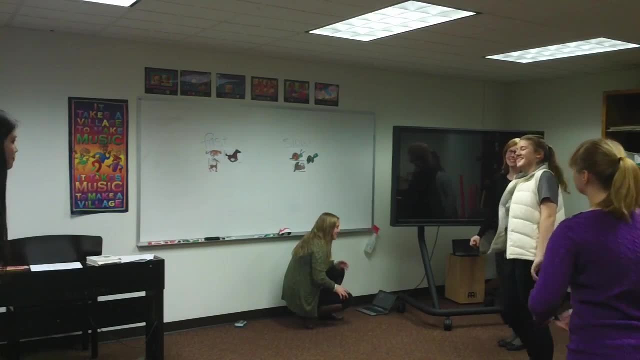 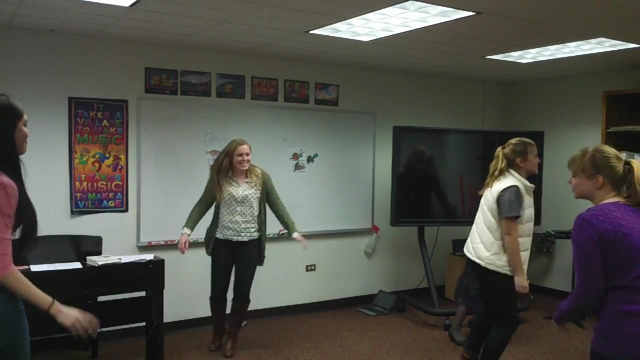 A frog, A bee, A bumblebee. This song is called Flight of the Bumblebees. Now, bumblebees move very fast, right Alright, let's try another one. I love this beat. Good job. 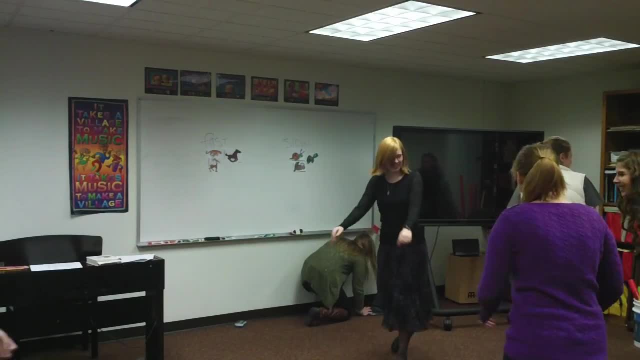 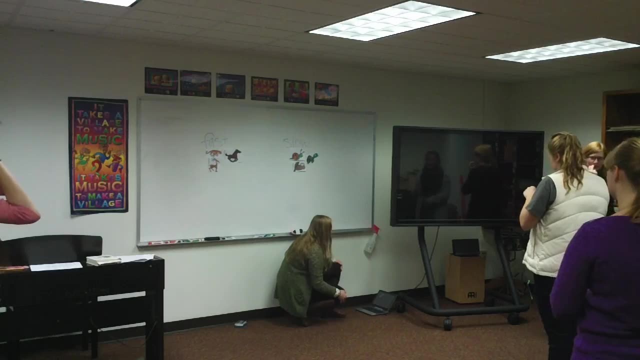 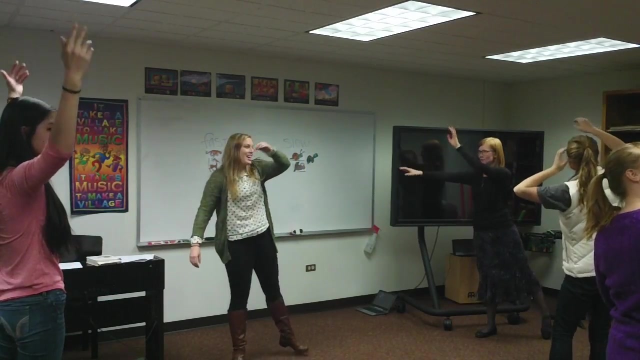 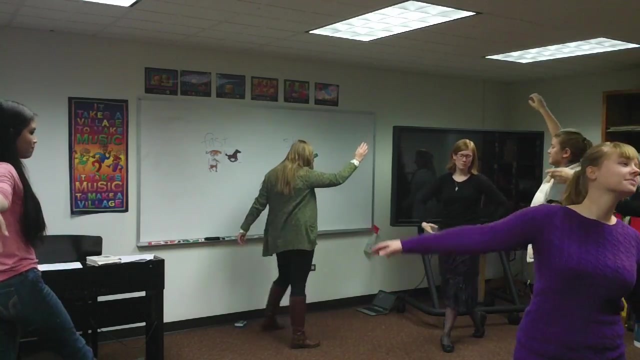 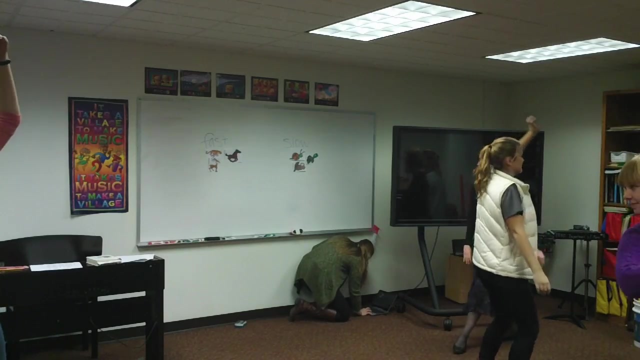 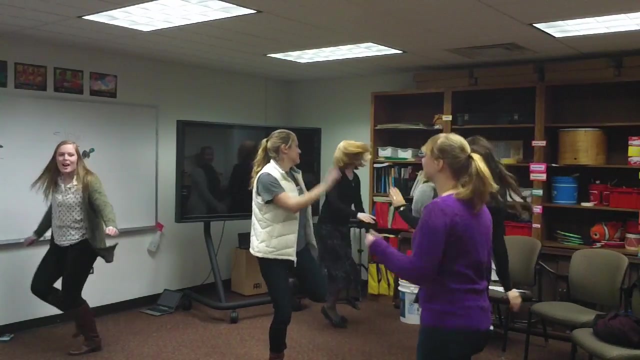 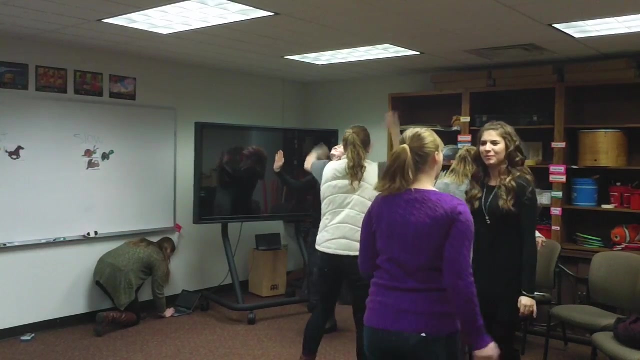 Very fast, very fast, Good job. This one's slow right, Very nice. We're going to do two more. Is this on fast or slow, Fast, Fast? Yep, Good job. Alright, on this last one, I want you to dance your way to your seats. 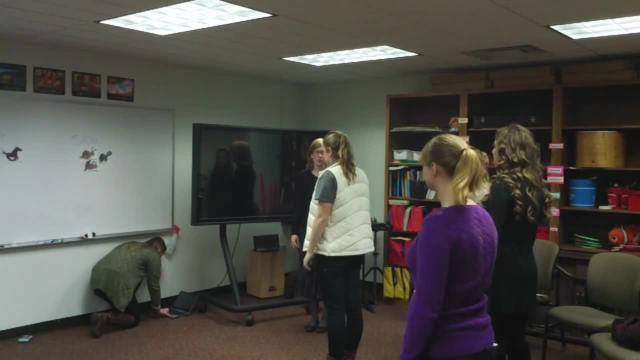 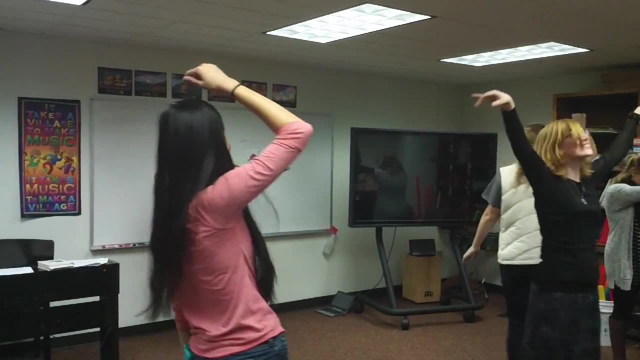 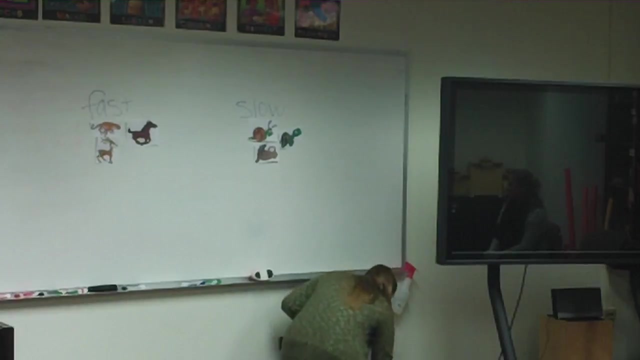 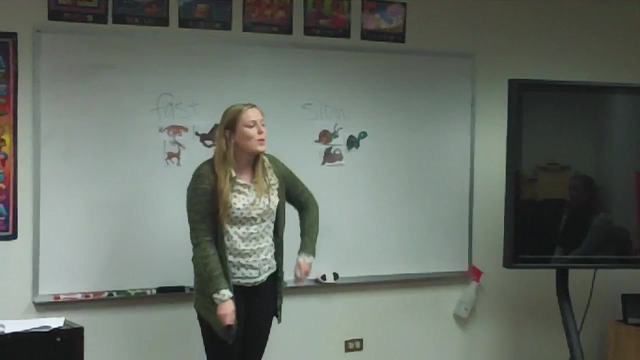 When you tell me whether it's fast or slow, Go ahead and dance your way to your seats- Good job. Now, that last one we did was that fast or slow, Slow, Slow. That was a great job. You guys got that all very quickly.